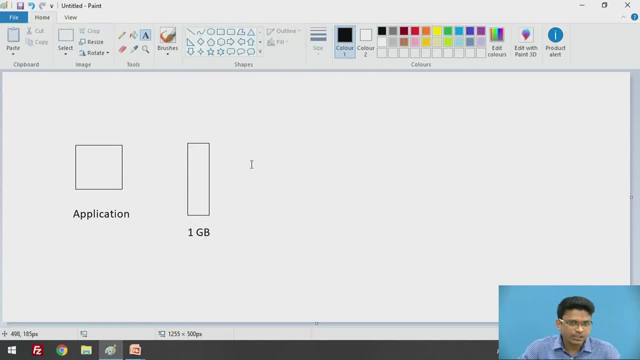 to double click or open that application, we need to place that application into the memory. So let's say we'll have one application and that application is needed two GB of the memory. So now, while performing these operations, it means while running that particular application. 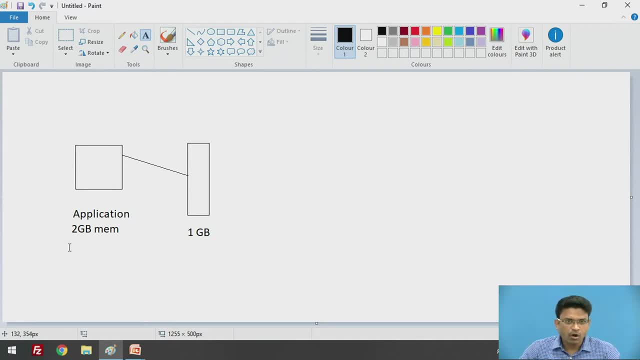 that particular application is needed as a two GB of RAM or memory. That is nothing but our logical address. So now, when that particular application is running, we need to place that application into our RAM And here we'll have that RAM with a memory. So let's say we're 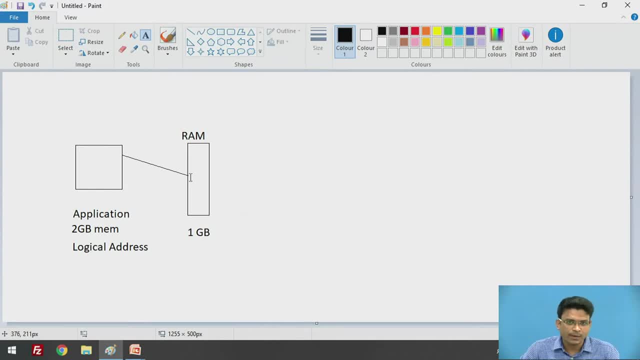 going to have one GB of memory. So now, while performing this operation, storing this two GB of RAM, two GB of application into the one GB of RAM is not possible. So now, this is nothing but our physical memory. So RAM is nothing but our physical memory. So now, 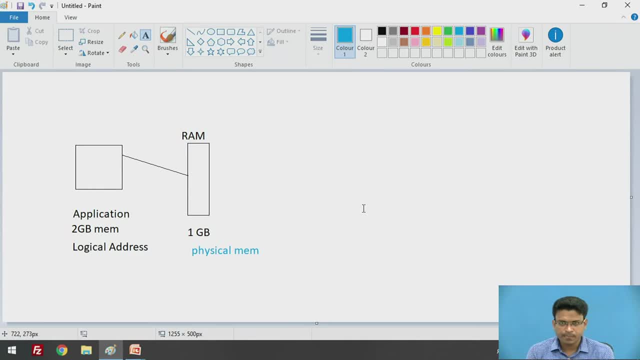 while performing this operation, then what the option will get then? So now, on the disk, we'll have this application Here, we'll have this disk. So now, in this disk we are going to execute that particular application. We have stored that application here. So now, whenever we'll install any operating, 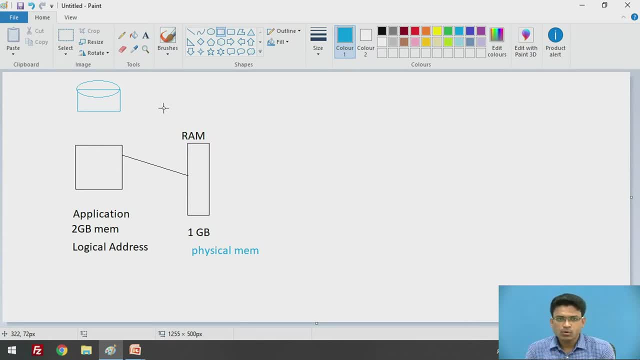 system. so at that time we need to keep some space free in C drive, D drive, anywhere where you have installed that particular operating system. Why? Because our operating system is going to use the version. So now, what is meant by virtual memory then? Alright, operating system is going to use. 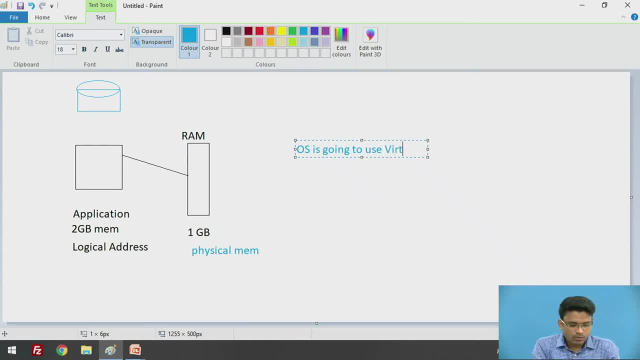 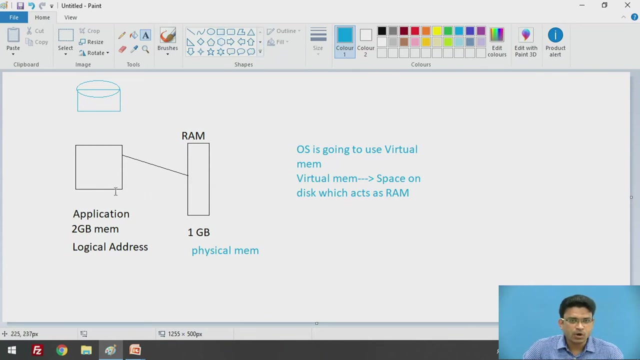 virtual memory, Then what is meant by virtual memory then? So the virtual memory is nothing but the space on disk which acts as a ram. fine, so means what if that particular application is not able to fit into this particular physical memory? so at that time we need to use this particular virtual memory. 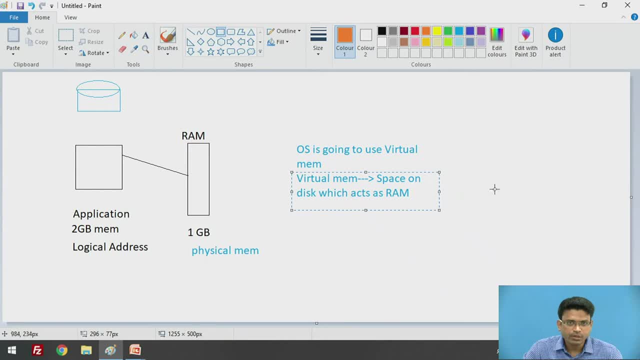 fine, we need to use that one. so now, how we are going to use that one then. so here that particular application need to use, let's say, on this disk. let's say this is our disk, so on this disk we'll have the virtual memory. so this is our virtual memory. let's consider this our 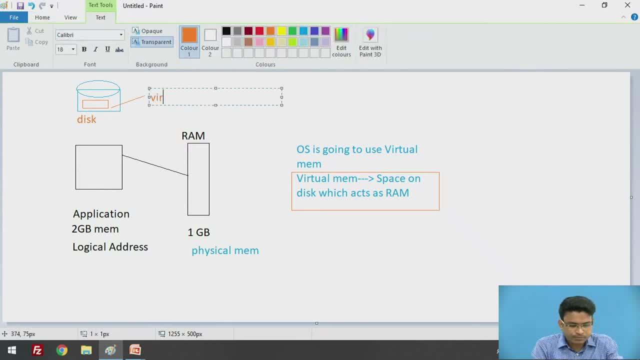 virtual memory. so now, on this virtual memory, we are going to load that application. so now, now here, we are going to load that particular application, this is our application, and this application we are going to load into that virtual memory. so now, how, in the which form, we are going to load that one, so to perform, 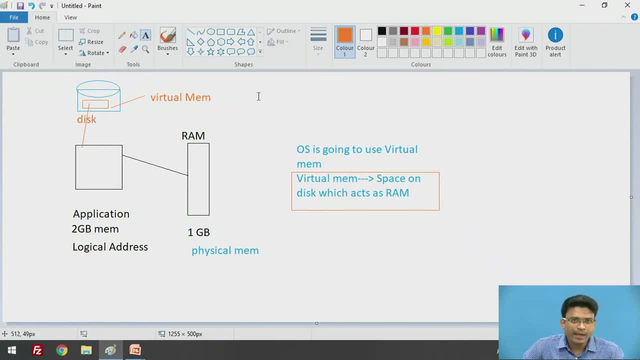 that what we need to do. we need to divide the application, divide application into pages, right? so now that particular application has been divided into the pages, and here we have loaded that particular application in the form of pages. right so now, whenever particular application is needed, let's say, now we got the what is the use of that particular virtual memory? right so that. 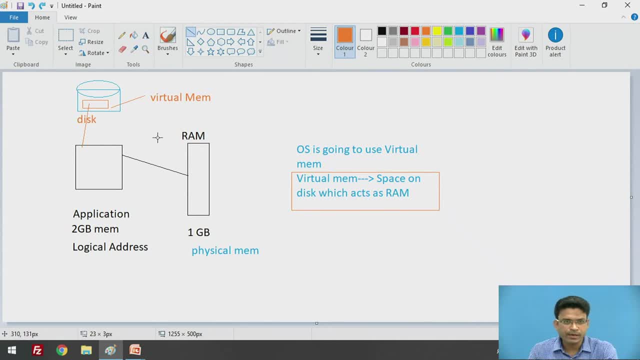 virtual memory is nothing but the space on disk which acts as a ram. fine, so now, currently here we'll have only one gb of ram, right? so now executing that much of may application- 2gb application- is not possible, right, when we can't load that 2gb of application. 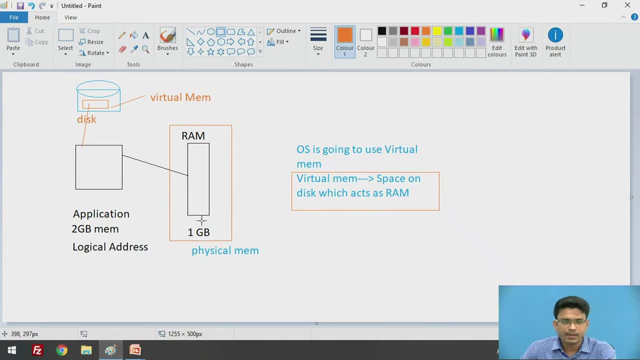 into the ram. so that's why we are going to use the virtual memory, right? so now, how we are going to utilize then that application is going to be divided into the pages, right? the application has divided into the pages, so now we are going to use those pages now. 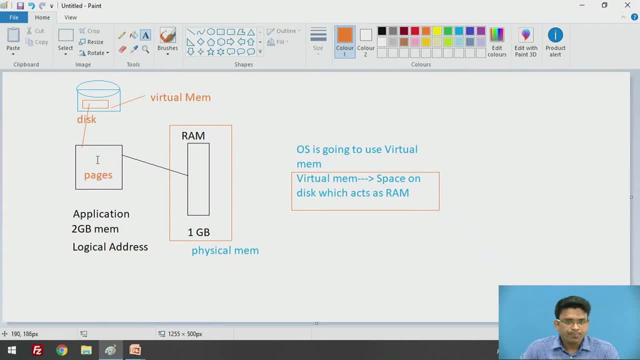 these are the pages, right? so these pages are going to be loaded there. so now say, we are going to teach you how to load these pages now, so later we are going to show you on how we are going to create videos with these looks after this particular problem. just see what. 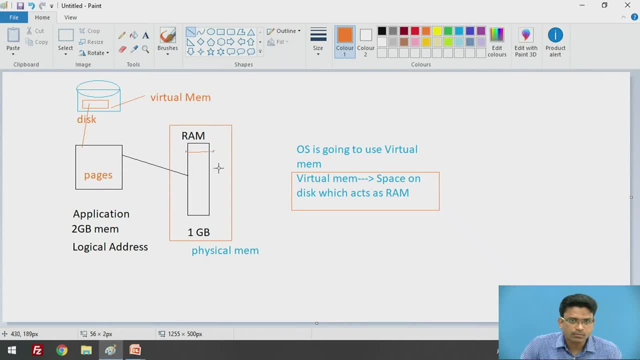 depends upon what accessibility the database is okay. how can you install, actually creating- and this may be your own thing- not getting copyright charge right now? if you download and you install gControl system, which of these three things? now we are actually not using these? the data Sprite support, Display, training function feature. so these database is now 그다음에. 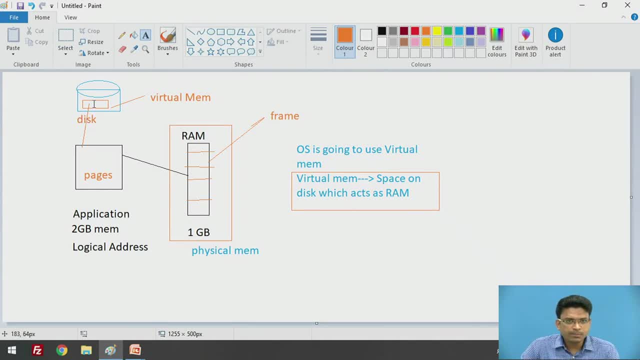 so now we need to load these pages into the frame on demand, right? so, basically, that is nothing but our virtual memory we have seen. so now let's discuss about the demand page, right? so let's discuss about this demand page. so now, what happens in a demand paging? so then, in demand paging, what we need to do that? 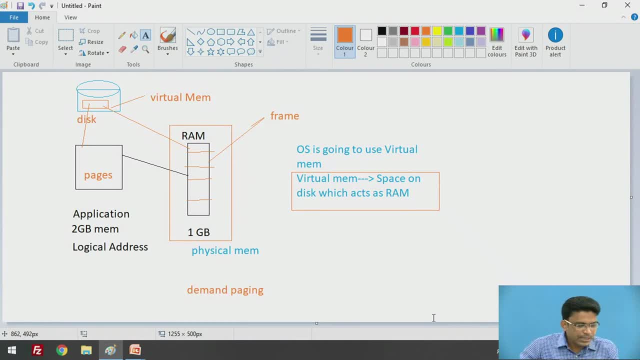 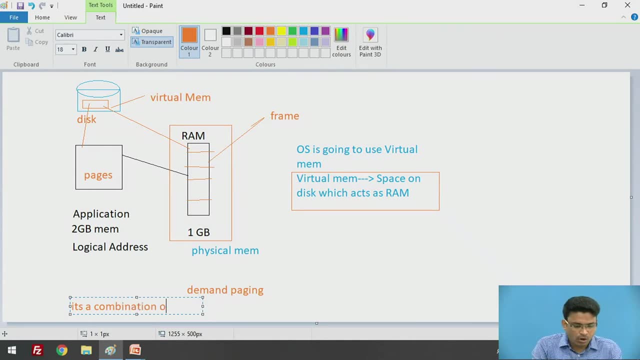 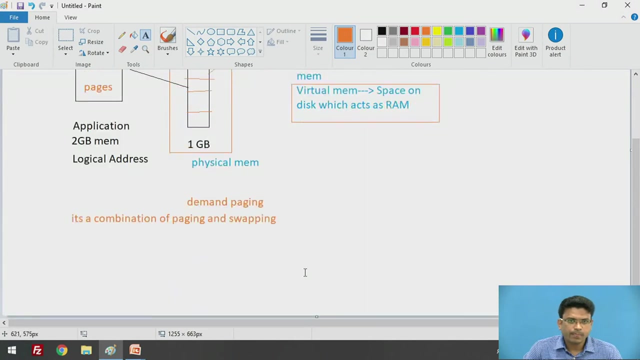 demand. paging is nothing but the combination of paging and swapping. fine, it's a combination of paging and and swapping, right, so how we are going to do that then? fine, so let's say, consider here again: paging is a concept, we got it. that page is nothing but the. 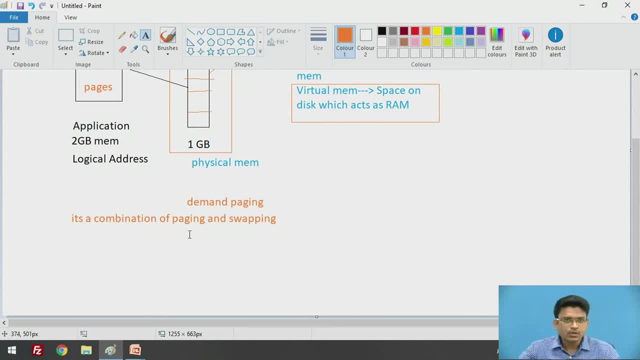 application is divided into the pages. so now, what is mean by then swapping? right? so now here, let's say we'll have our disk, fine, this is our disk. so now, in this disk we'll have the pages. fine, hmm, we'll have small, small pages, right, those applications are divided into the 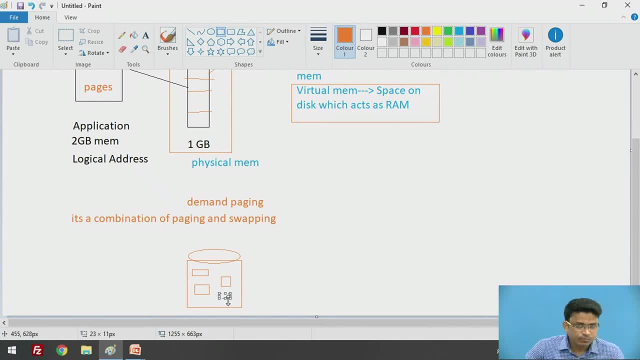 pages. fine, so let's say, these are our pages. so now, while performing this nine, now here will have our RAM. fine, this is our RAM. so now, this RAM has been divided into the frames. right, so now, while performing these operations, right, while performing these applications, right, so say in this: 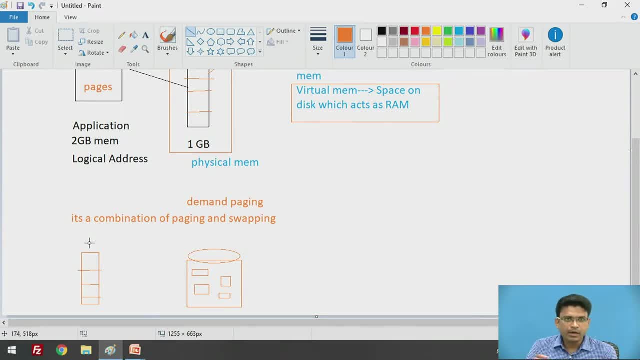 particular예요, terminate server paging. in the same way, while performing the applications, right, so say, in this particular particular RAM, currently one application is running, So now that application is running and some part of that application is stored in the disk, right, Because we are going to 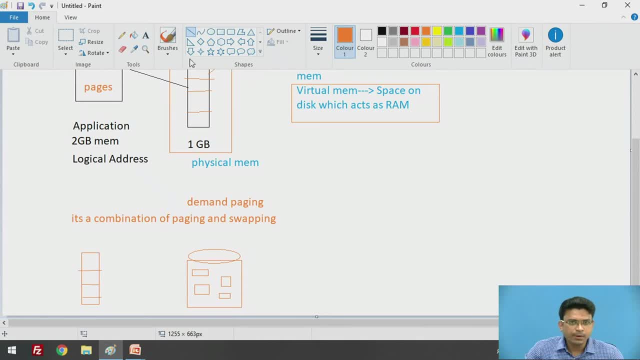 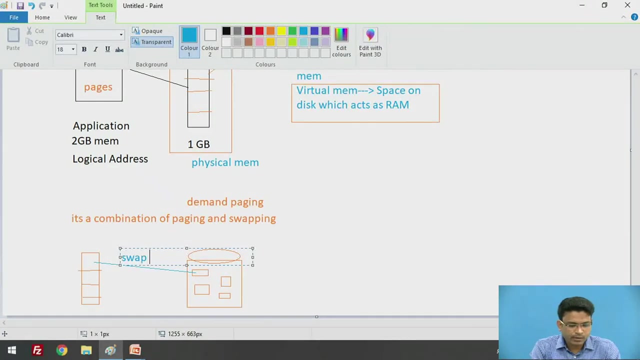 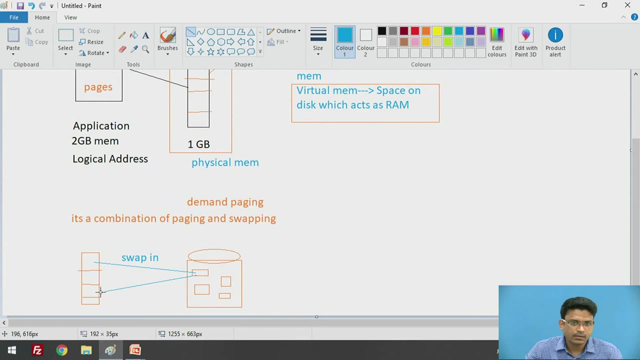 use the virtual memory. So at that time this particular application is demanding for some pages from the disk right. Let's say he wants to access this page right. So now, at that time we need to perform swap in and swap out operations. All right, Fine, Swap in and. 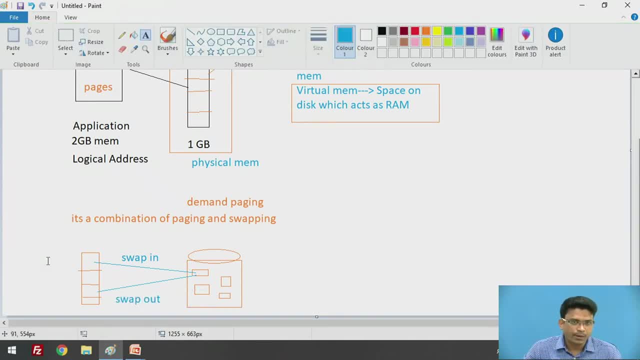 swap out two operations right. Why? Because some part of the memory is in the disk and some part of the memory is in the RAM. So on the other hand, we need to perform swap in and swap out operations. So at that time, 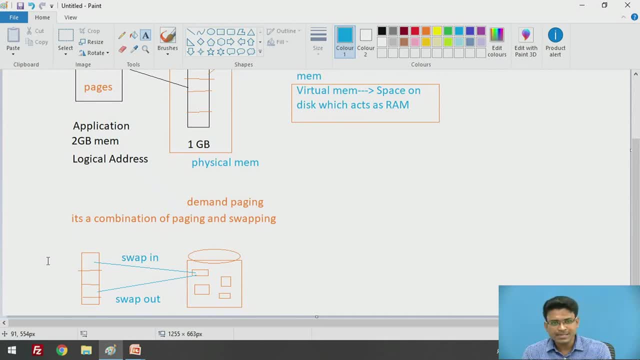 On demand, we are going to load the pages into the RAM by performing swap in and swap out operations. Swap in means what We are going to take that particular page from the disk into our main memory and after completion of that task, then we are going to release that particular frame. 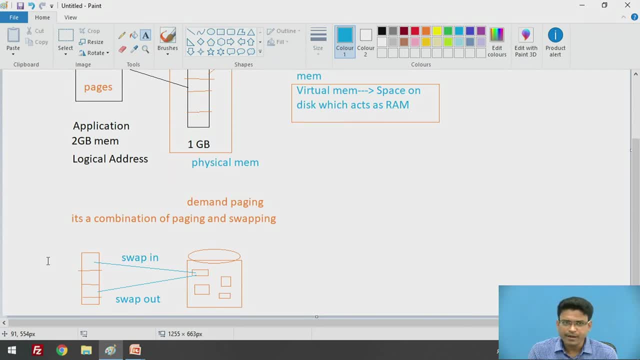 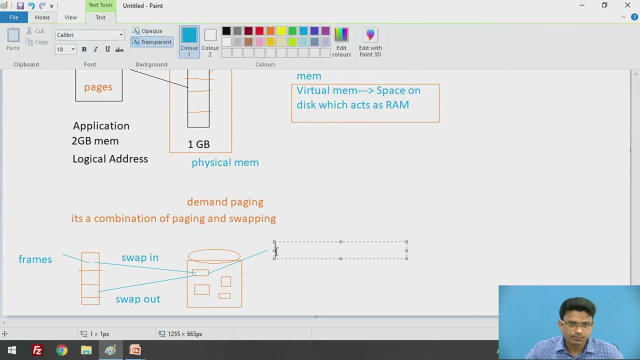 So, if you see this diagram, what we are getting is: these are nothing but our frames, right Means what We are going to store the pages into the frames, right, And these are nothing but our pages, right? So these are nothing but our pages. 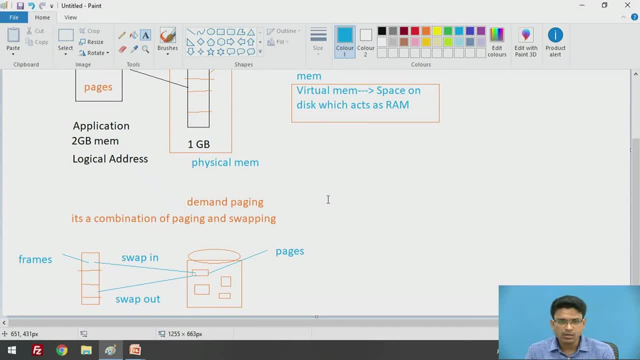 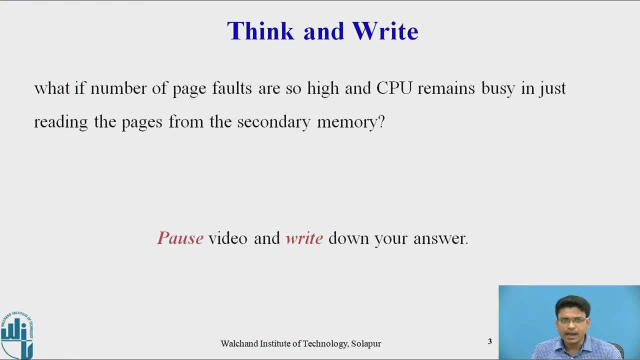 So on demand, we are going to perform this operation. So that's it. That's called the demand paging, fine, So we have seen both of the things. So let's think and write. What if the number of page faults are so high and CPU remains busy in just reading the pages? 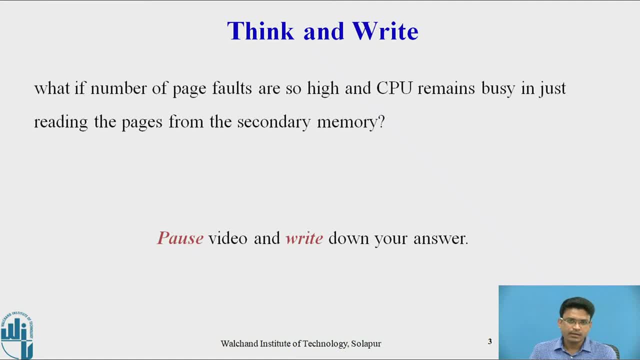 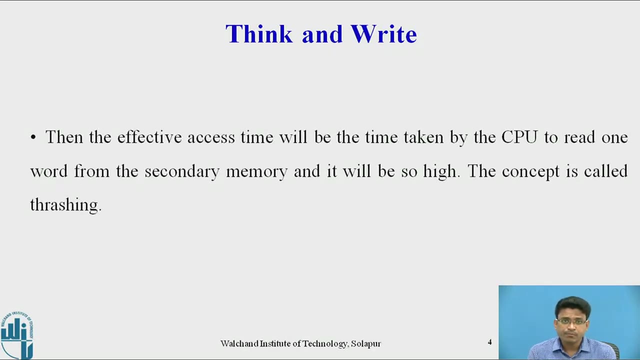 from the secondary memory. What happens? Just think on this. Let's see. Then the effective access time will be taken by the CPU and read one word from the secondary memory, and it will be so high That concept is going to be called thrashing right.